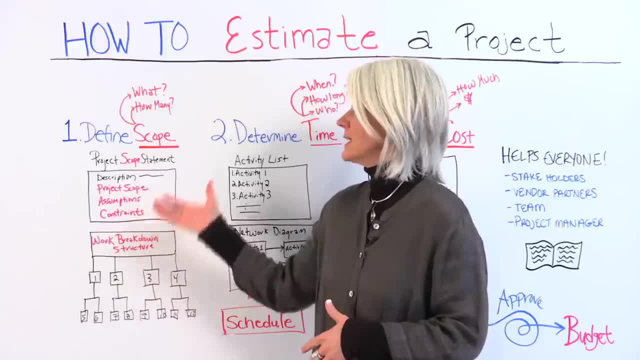 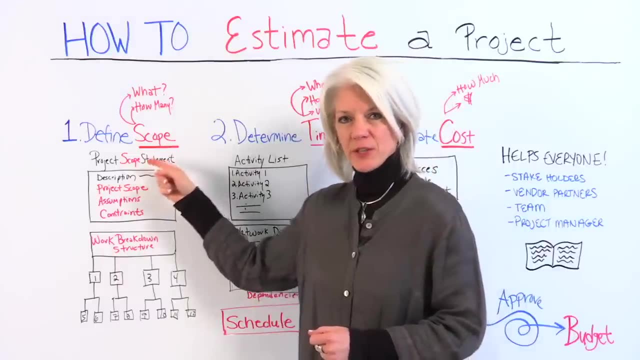 we're talking about. what is this project? What are we producing? How many are we producing? This is defined in our project scope statement, which is a description of the scope, And it also outlines again what's in the project and what's out of the project. It also includes: 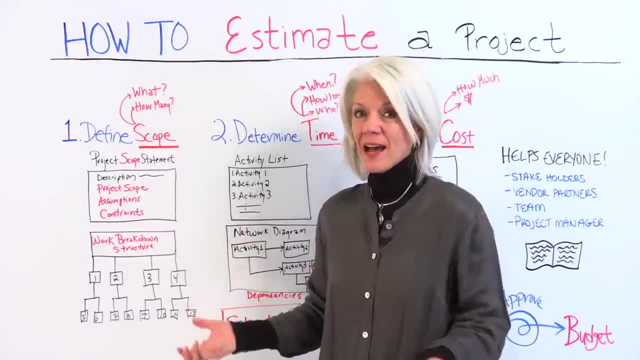 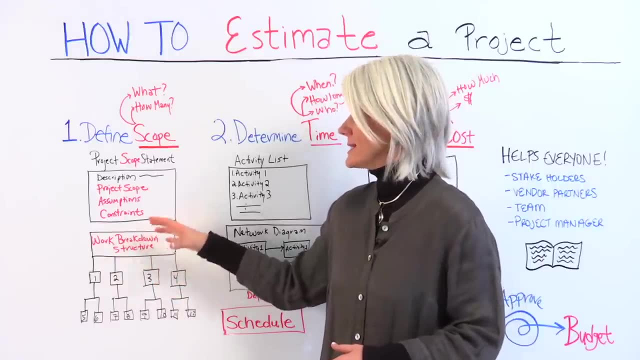 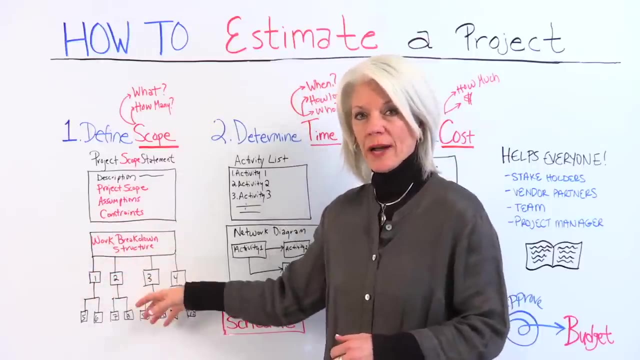 assumptions and constraints that may or may not impact the scope. The scope also has the work breakdown structure, which breaks down all of the work of the project in the more detail. The more detail we can get the work required then the better estimate that we 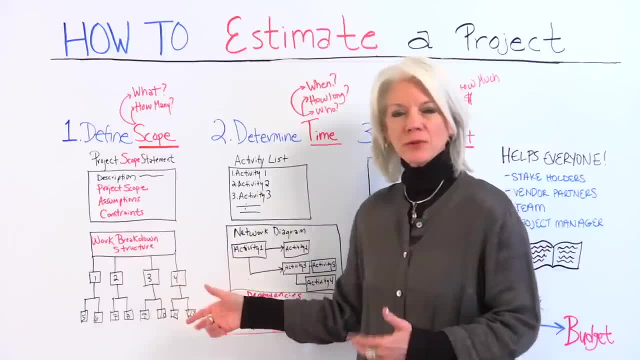 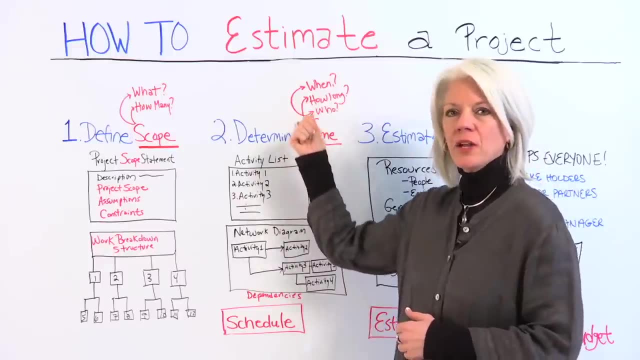 can build. So the work breakdown structure is also used to determine the time it's going to take to do the project. So when we talk about time, we're talking about when are we going to get this done, how long is it going to take and who do we need to get this done? 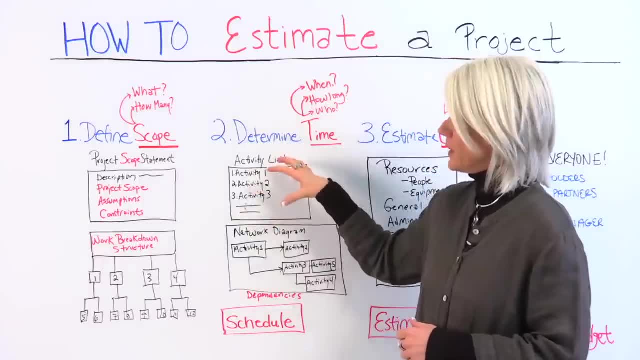 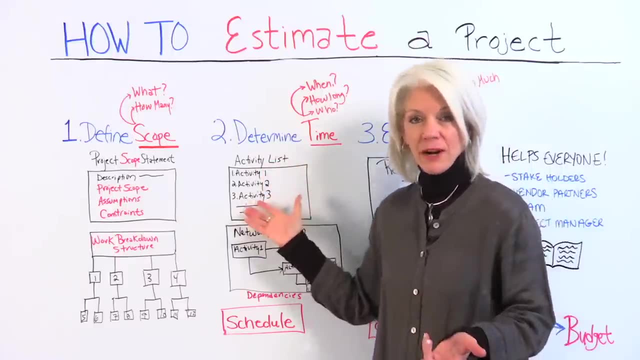 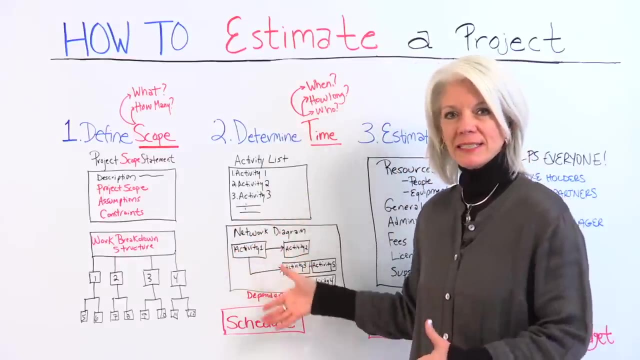 So when we get the work breakdown, structure and the scope, it helps us to create an activity list. So the activity is breaking down all the activities required in the project And that is used to help build a network diagram. So with the network diagram and the dependencies, 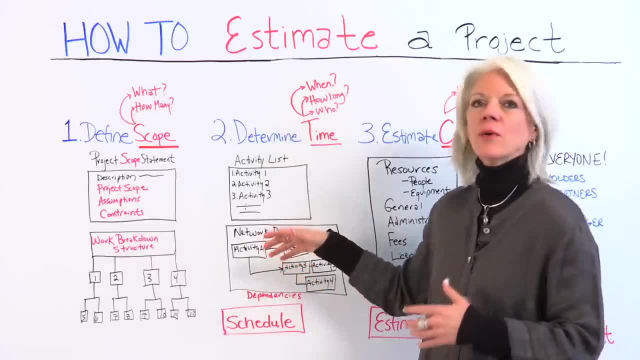 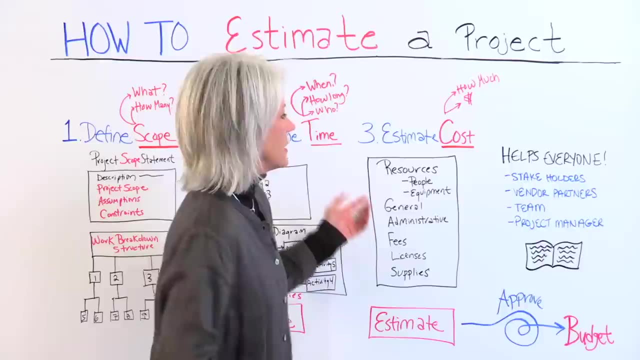 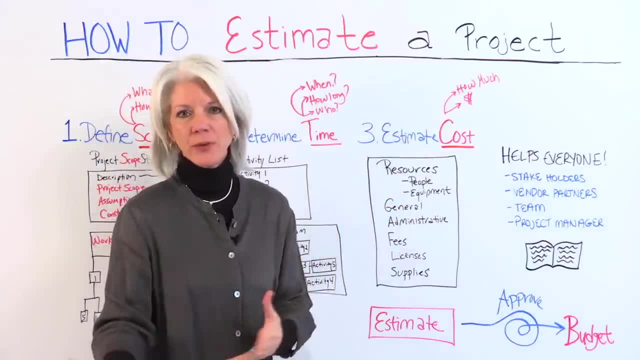 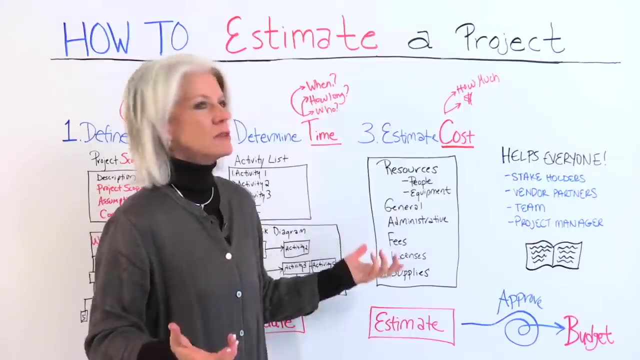 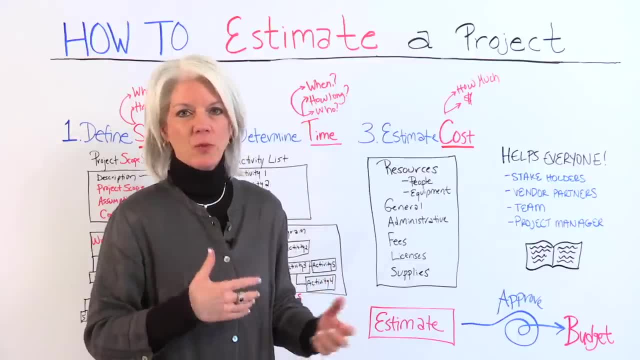 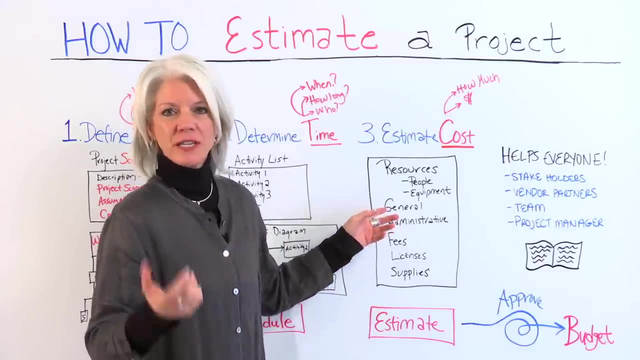 It also includes equipment. Do we need any equipment And what kind is it? Where does it come from? Where does it ship, Which could impact the cost? It also includes general cost of the project. It could include administrative cost or it. 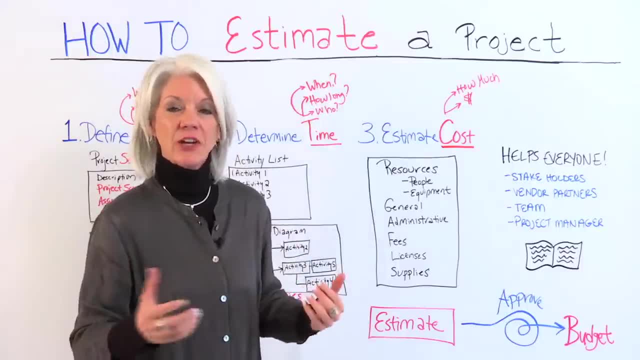 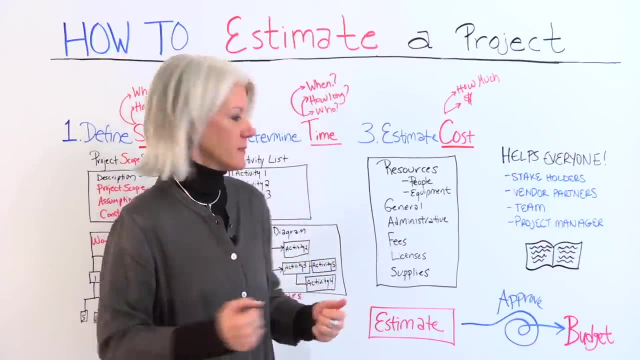 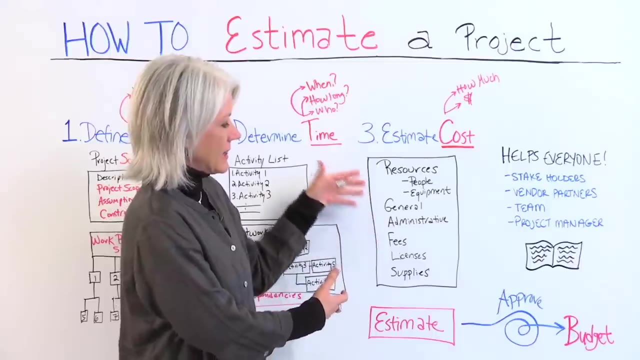 could include any kind of fees or penalties or bonuses. It could include commissions. It could also include things like licenses, maybe any kind of rent. It could also include supplies we may need. So you can see the long list of cost we take and that becomes now.